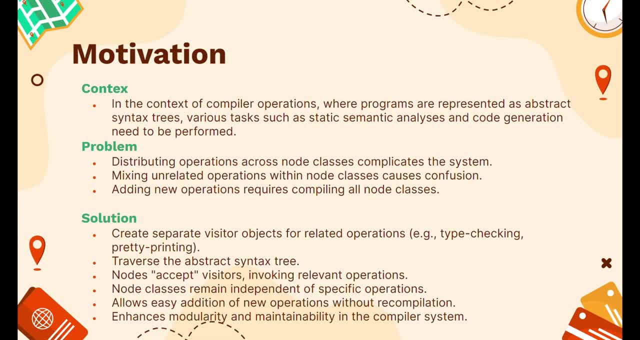 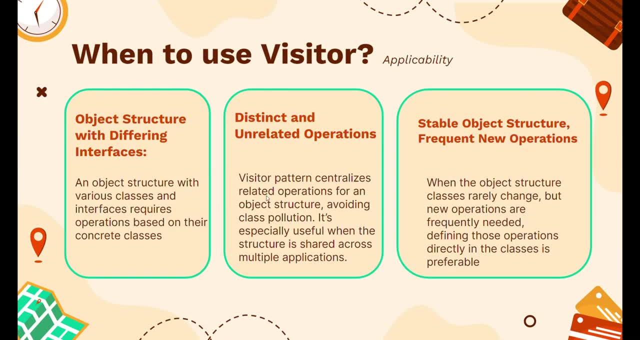 Ultimately, it enhances the modularity and maintainability in the compiler system. So when do we use visitor? We use visitor pattern when we're handling the operations on objects in the object structure with varying interfaces based on the concrete classes. We employ the pattern when made distinct and unrelated operations must be performed on objects to prevent cluttering the classes. 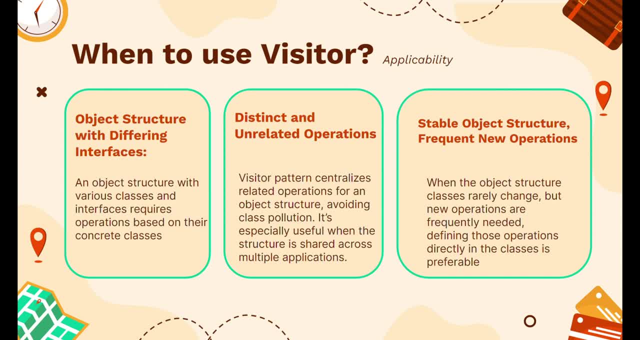 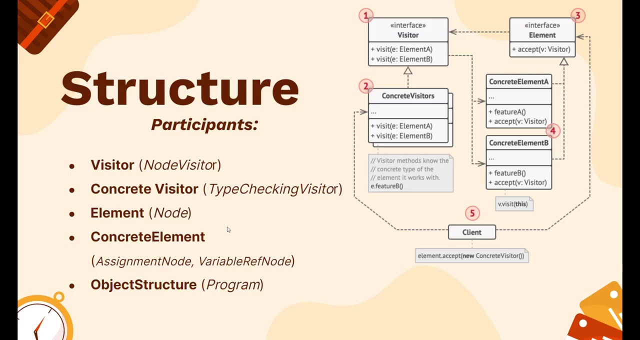 And we consider using the visitor when the object structure remains stable, but new operations need to be frequently defined. If the structure changes too often, it may be more efficient to define operations within the structure classes. This is the structure We have: the participants of visitor. 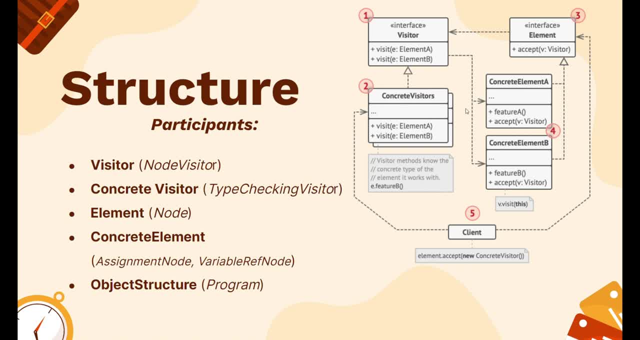 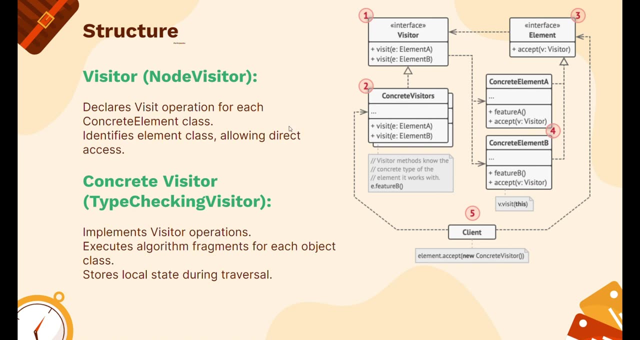 The concrete visitor, The concrete elements, The elements And the object structure, which is the application We have. the visitor declare visits, operation teller to each concrete element, class, Discern the specific class of the visited element And accesses elements via their specific interfaces. 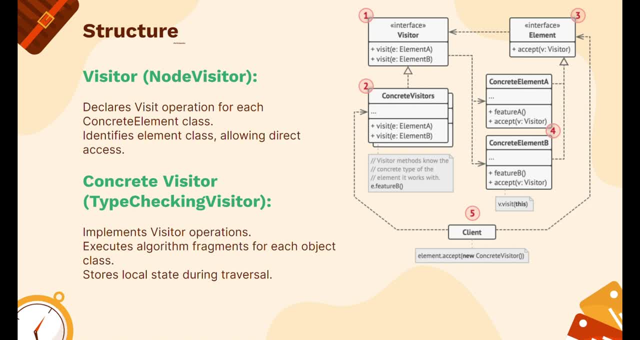 The concrete visitor implements the visit operations specified by visitors. executes algorithm corresponding to object classes and maintain the local state of to the accumulate traverse results. The element divide and accept operation facilitating visitor acceptance. The concrete element implements the accept operation permitting visitor interaction. 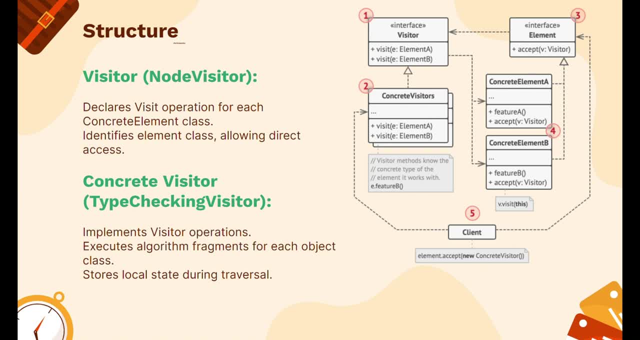 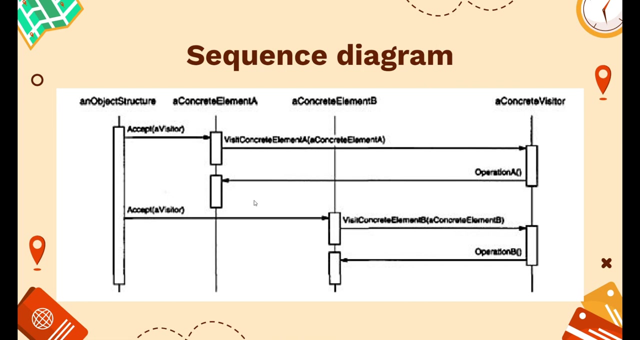 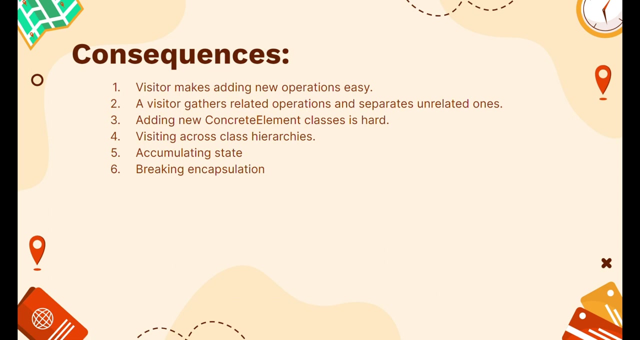 The object structure, which is the main, emulates the elements, furnishes and traverse, a traversal interface for visitors, and may adopt a composite or collection of structures. This is the sequence diagram of the class diagram. For the consequences, The visitor pattern make it easy to add new operations to complex objects without changing the classes. 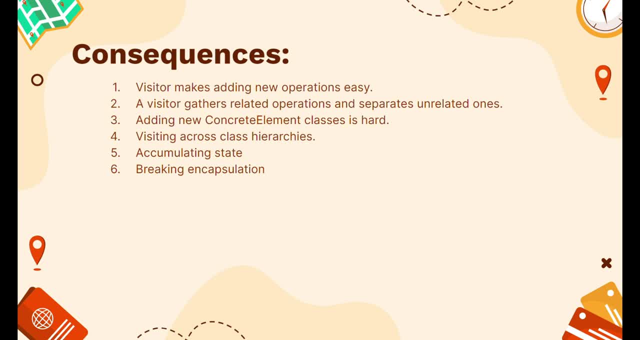 It gathers the related operation in the visitor classes, simplifying both elements and algorithms. However, adding new types of elements can be difficult And this may not be suitable of if elements classes change too frequently. Visitor can traverse different types of object structures. 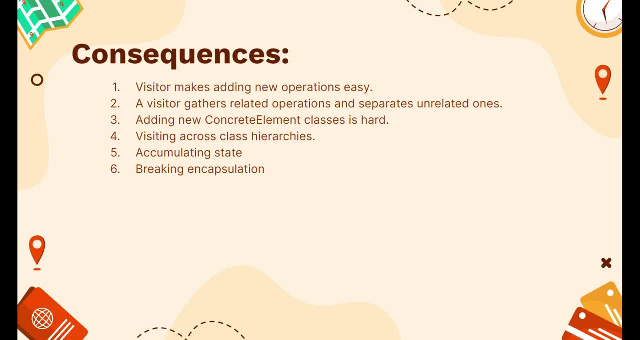 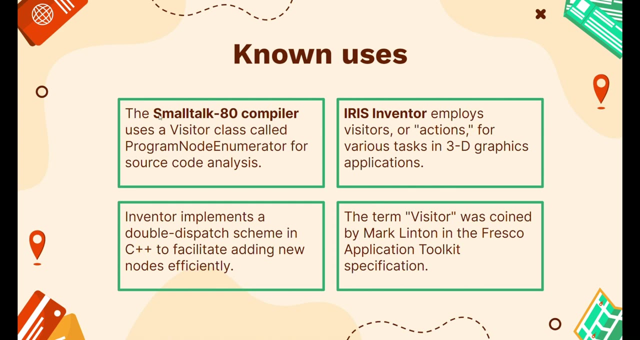 This accumulates state but may compromise encapsulation by requiring public access to the internal states. Some of the known uses from The book are: the small talk 80 compiler. The iris inventor, which is the Um, Is employed. visitor for actions for the various tasks in 3D graphic application. 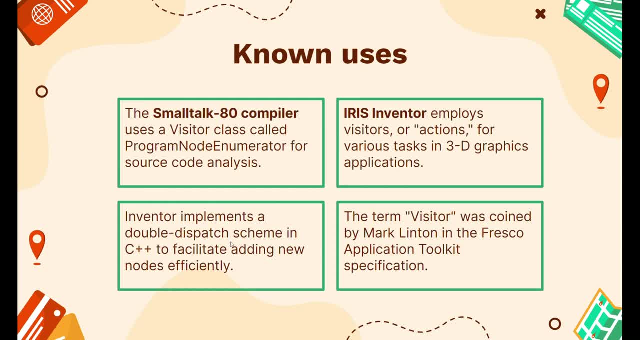 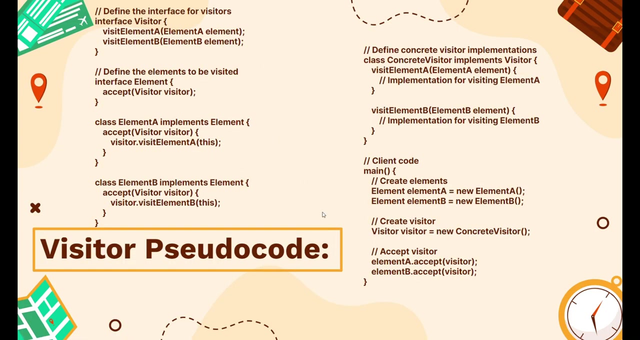 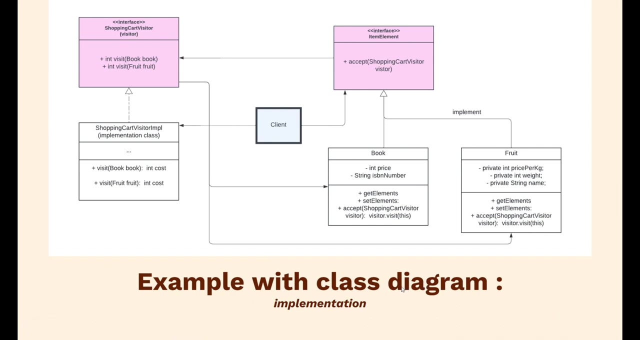 The um, the inventor, also implement a double dispatch scheme in the C++ To make adding new notes more efficiently And Fresco application to kids. This is a pseudocode for um implying or applying the visitor behavior Pattern. This is my example class diagram. 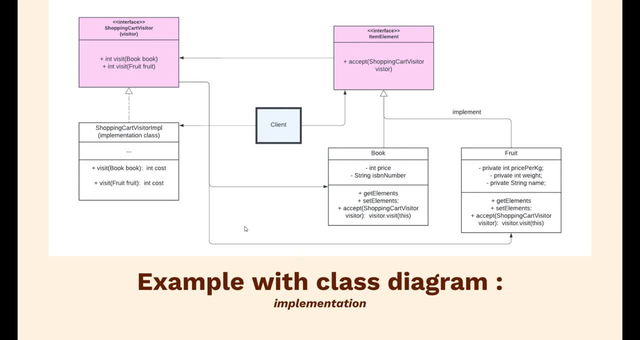 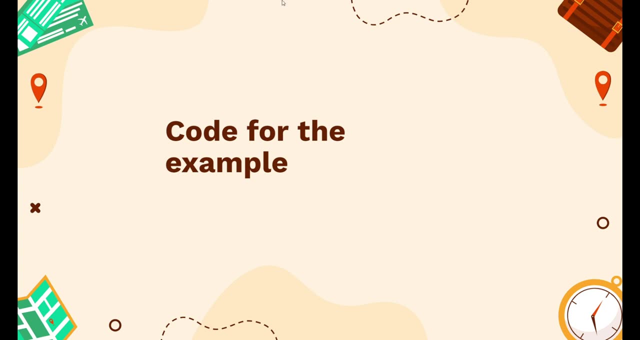 From for um The shopping cart visiting Which contain the? um contain books and fruits, And this is example of my code. We have the client, The items Of, With a element with the interface And this is the visitor. 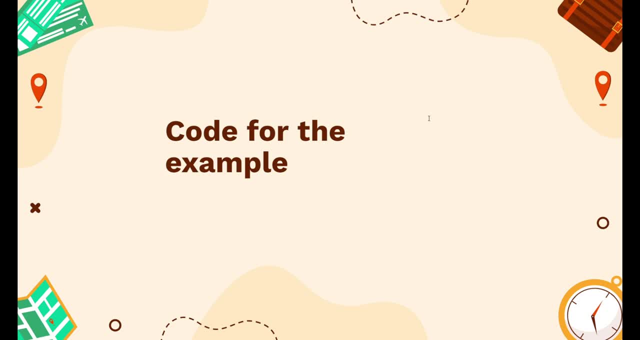 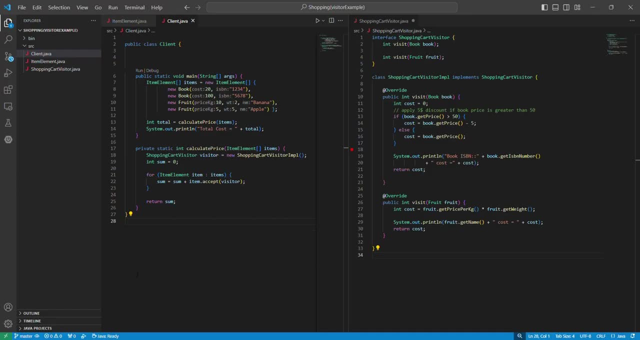 Let's run, And this is my code Example. We have The Um The client, Which is the Um I'll A lot Of the client, So um, And that is The I'm not. 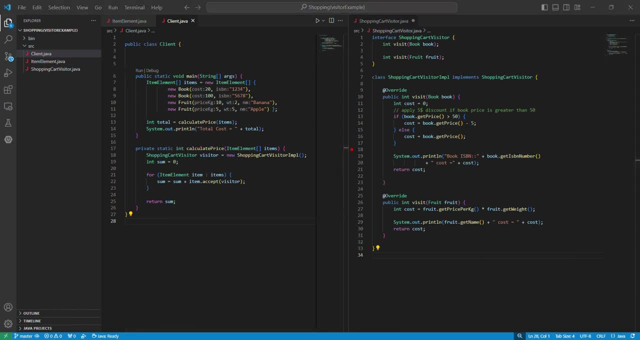 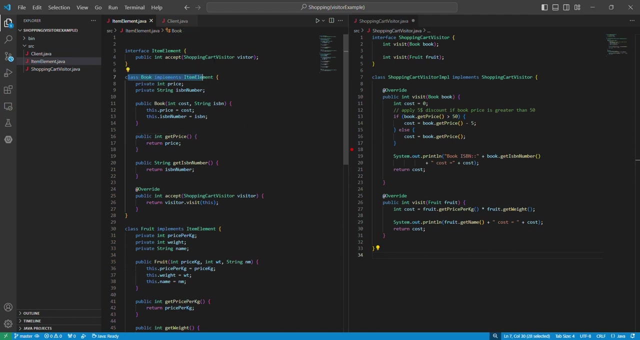 Do Yeah, Oh, One, Uh, So uh. the object structure of the program. We have the concrete elements of fruits and book with the interface of the item element. Then we have the visitor, which is an interface: interface with the concrete visitor. 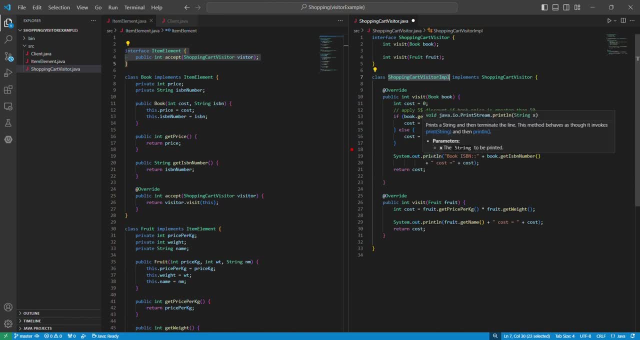 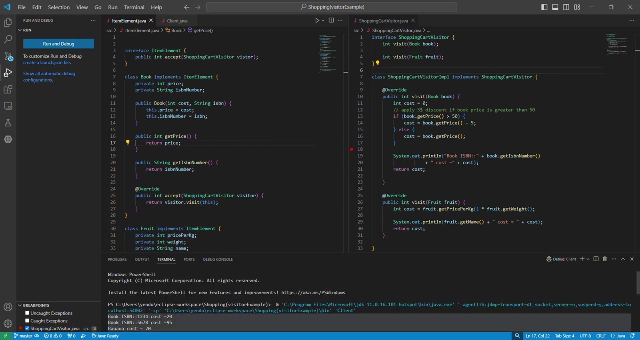 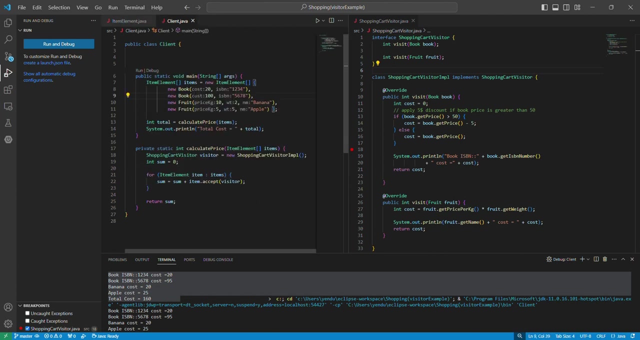 of the shopping cart. visitor implementation Info. is implementation Now. let's run it Now. we see when the client adding the books and the fruit into the cart- when I want to do that, whatever more than $50, the book gonna get discount. 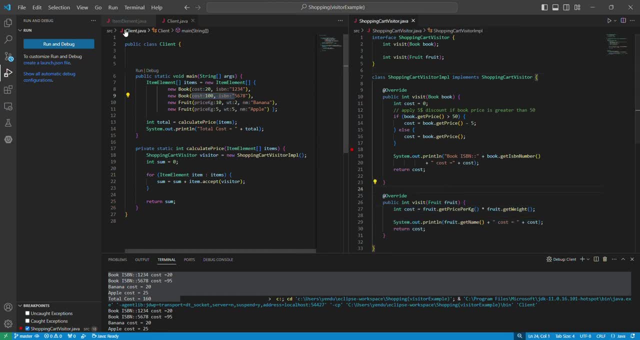 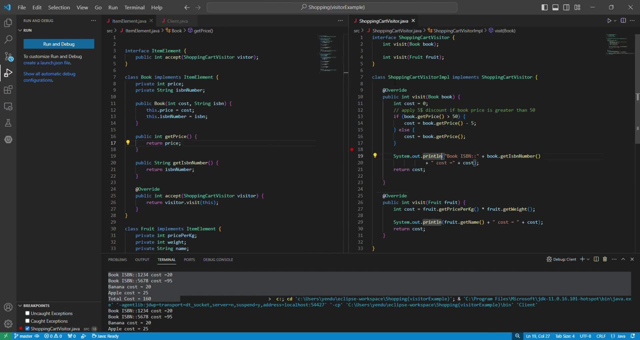 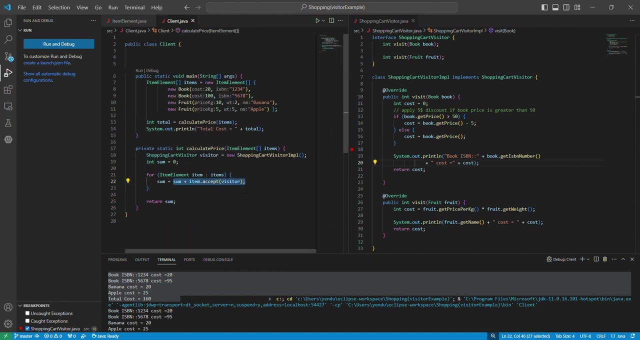 Why I don't want to do the same with the fruit. So I take them the functional and make it the external class in the, so when the client at the element is will also get when we do the sum into the accept of the visitor. 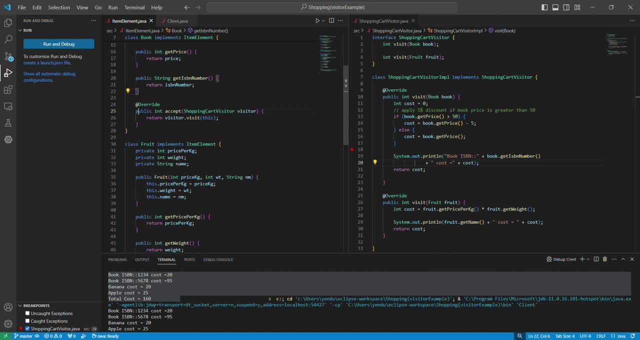 they will go inside here And check with the accept function or accept method, which is we'll get override and check inside here of the shopping cart visitor implementation. Then is we'll do external, externally here, checking for the cost and whatever. whatever book that is more than $50 gonna get discount.